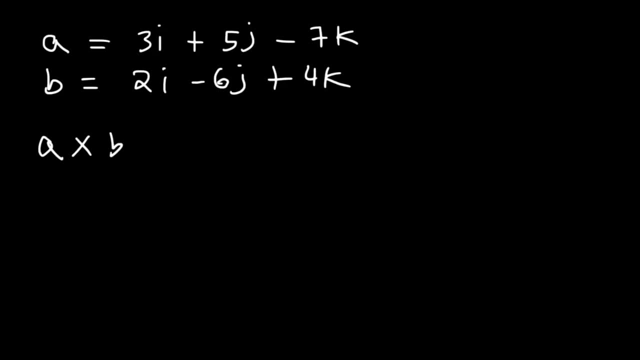 So what is the cross product of vectors A and B? How can we find the answer? 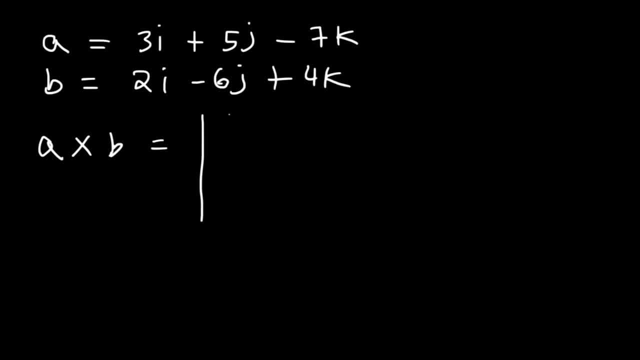 What I'd like to do is first put this in the form of a matrix. This is i, j, k, which corresponds to the x, y, and z components of a vector. And then first we need to put vector A in the middle, because that comes first. So it's going to be 3, 5, and negative 7. And then vector B, which is 2, negative 6, and 4. 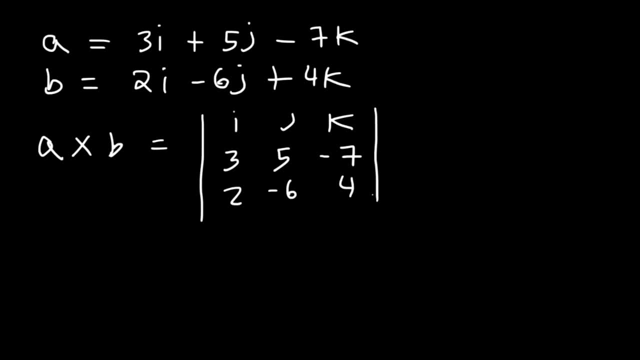 And basically, you've got to find... Find the determinant of this 3x3 matrix. So it's going to equal i. 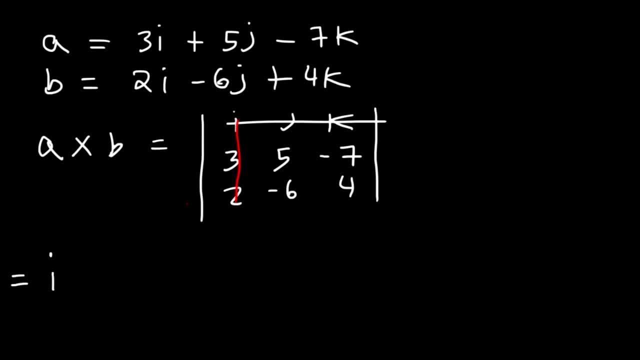 i is found in row 1, column 1. And it's going to leave behind a 2x2 matrix, highlighted in that red box. 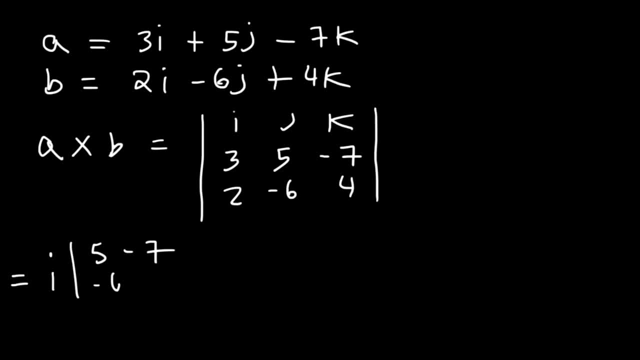 So that's 5, negative 7, negative 6, and 4. And then it's going to be minus j. 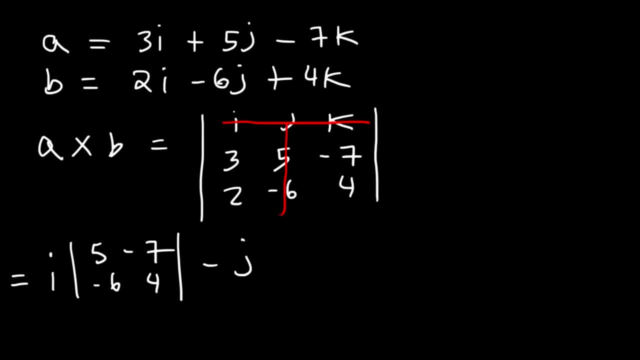 Now j is in the first row. Second row. Second row. Second column. 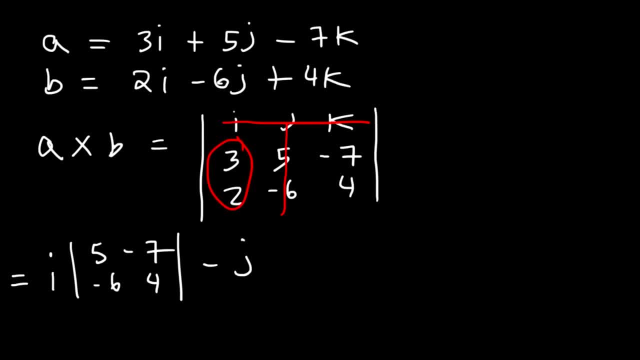 So we have left over 3, 2, and negative 7, 4. Next, we have positive k. 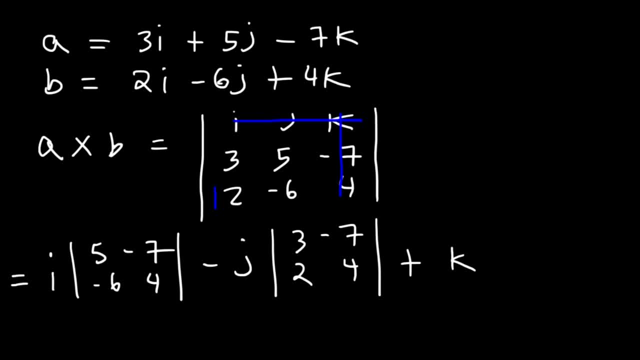 And k is in the first row, third column, which leaves behind 3, 5, and 2, negative 6. So this is what we know. And now we have... 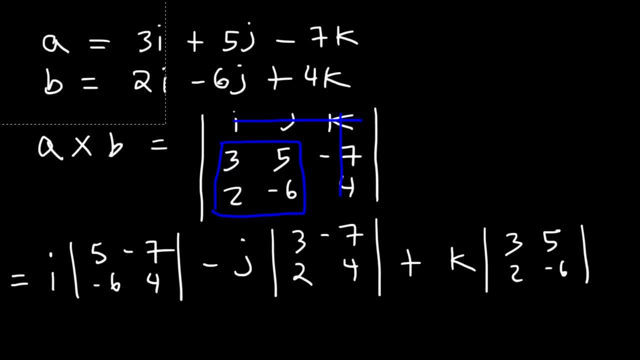 Now the next thing that we need to be able to do is to evaluate or find the determinant of a 2x2 matrix. 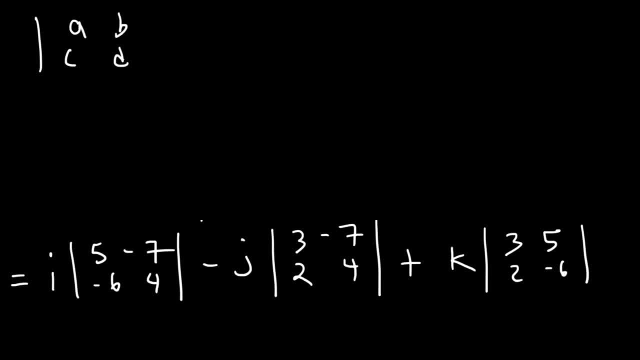 So let's say this is a, b, c, d. 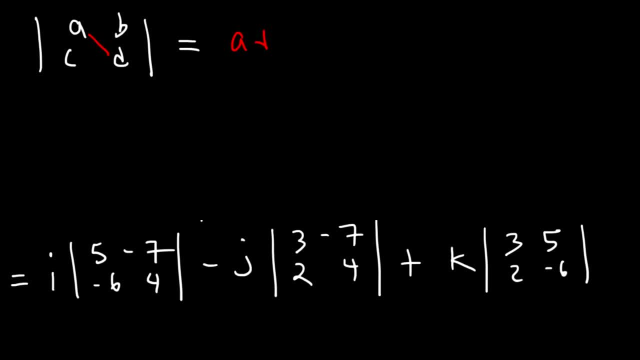 It's going to equal the product of a, d, minus the product of b, c. So that's how you can... You can evaluate the determinant of a 2x2 matrix. 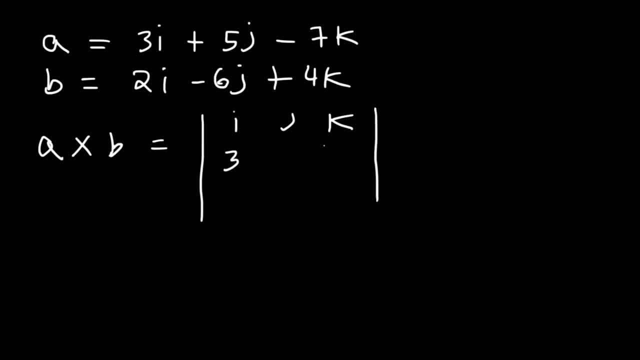 And then first we need to put vector A in the middle because that comes first. So it's going to be 3,, 5, and negative 7.. And then vector B, which is 2, negative 6, and 4.. 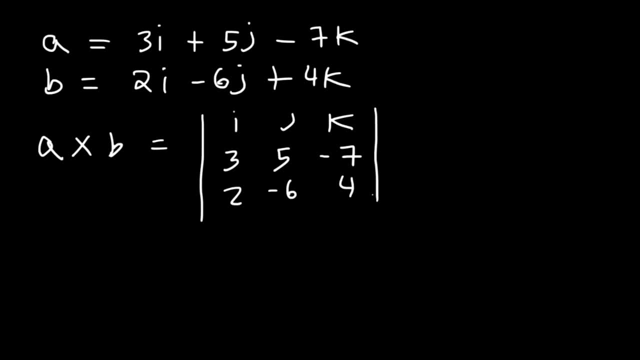 And basically you've got to find, Find the determinant of this 3x3 matrix. So it's going to equal i. i is found in row 1, column 1. And it's going to leave behind a 2x2 matrix, highlighted in that red box. 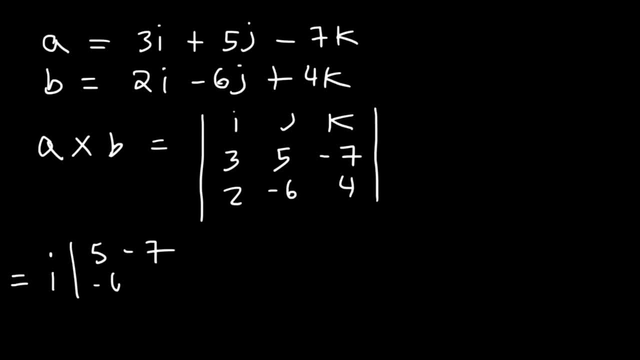 So that's 5, negative 7, negative 6, and 4.. And then it's going to be minus j. Now j is in the first row, Second row, Second row, Second column. So we have left over 3, 2, and negative 7, 4.. 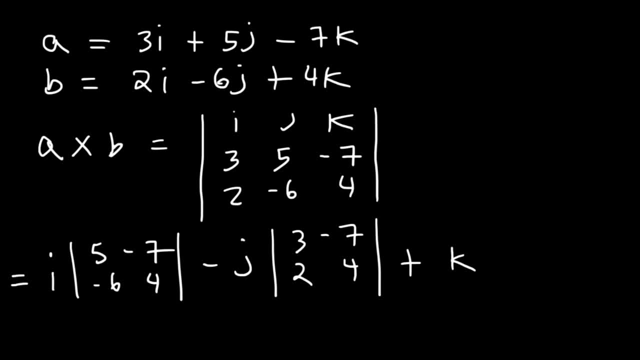 Next we have positive k, And k is in the first row, third column, which leaves behind 3,, 5, and 2, negative 6.. So this is what we know And we now have. Now the next thing that we need to be able to do is to evaluate or find the determinant of a 2x2 matrix. 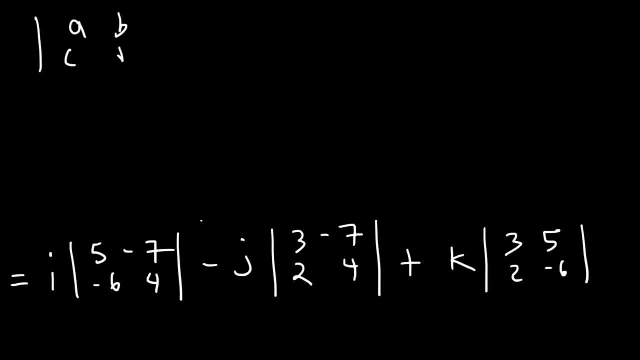 So let's say this is a, b, c, d, It's going to equal the product of a, d minus the product of b c. So that's how you can- You can- evaluate the determinant of a 2x2 matrix. 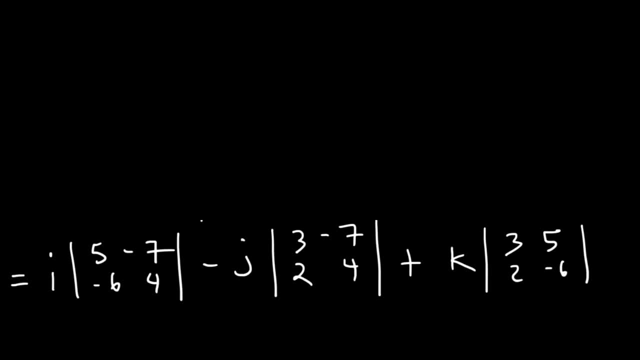 So let's do that for each of the 2x2 matrix that we see here. So the first one, it's going to be 5 times 4, which is 20.. And then, minus negative, 6 times negative, 7,, that's positive, 42.. 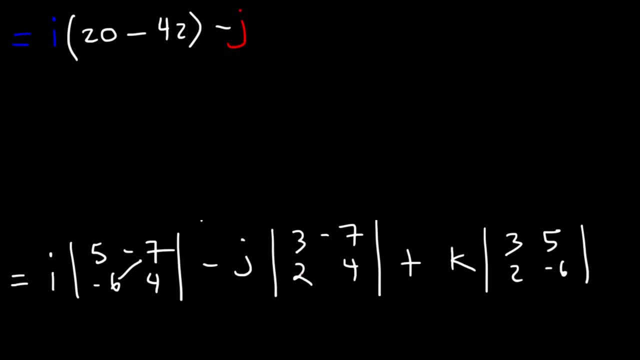 And then we have minus j, And then 3 times 4. That's 12.. Minus 2 times negative 7,, which is negative 14.. And then we have k: 3 times negative. 6 is negative 18.. 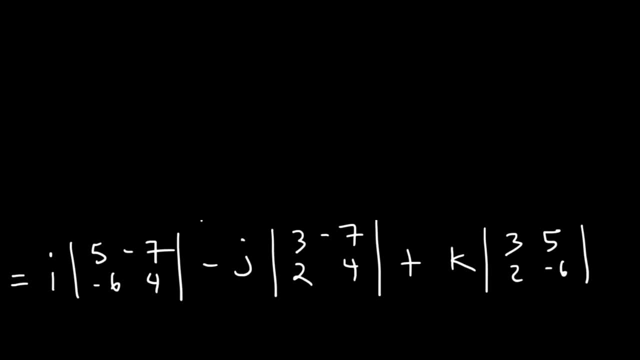 So let's do that for each of the 2x2 matrix that we see here. So the first one, it's going to be 5 times 4, which is 20. 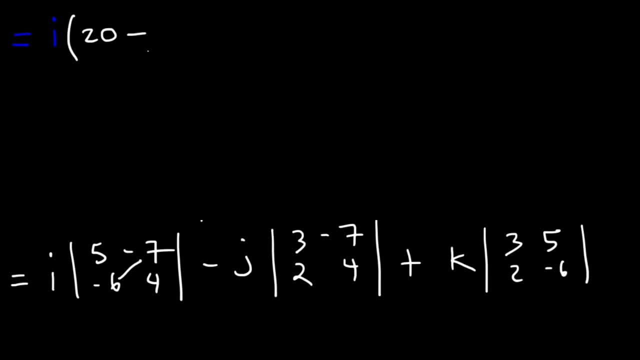 And then minus negative 6 times negative 7, that's positive 42. 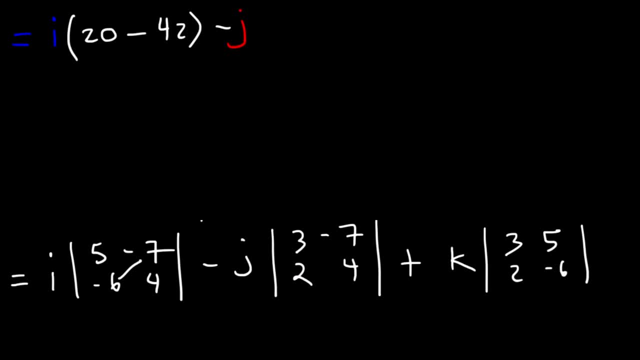 And then we have minus j. And then 3 times 4. That's 12. 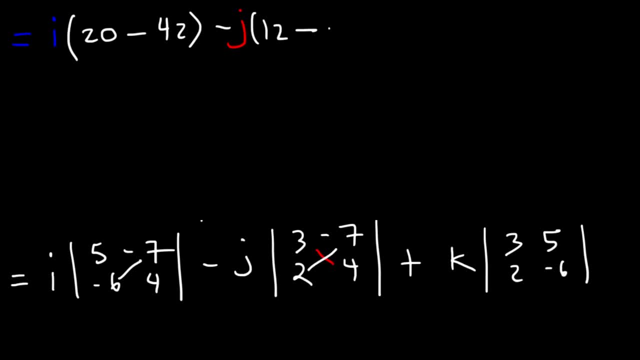 Minus 2 times negative 7, which is negative 14. And then we have k. 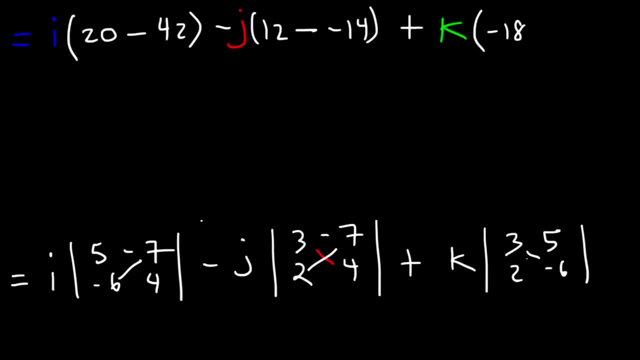 3 times negative 6 is negative 18. 2 times 5 is 10. So it's minus 10. 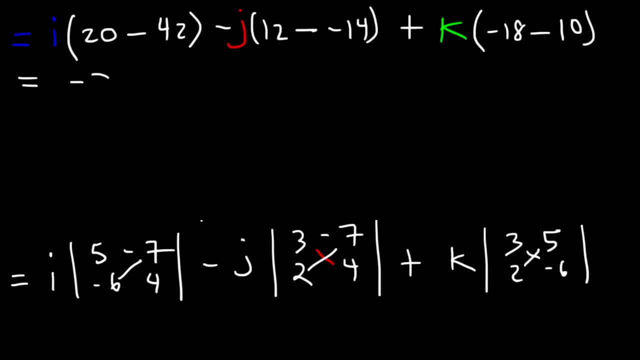 Now 20 minus 42. That's negative 22. So it's negative 22i. 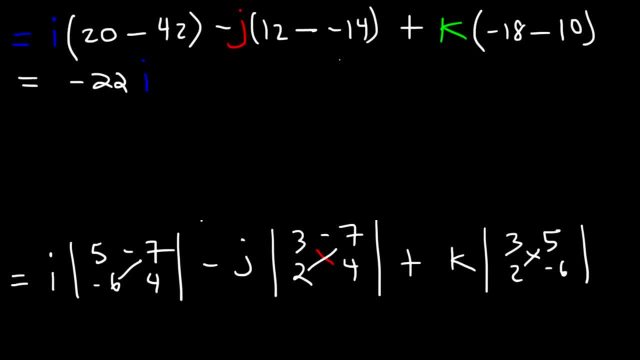 And 12 minus negative 14 is like 12 plus 14. 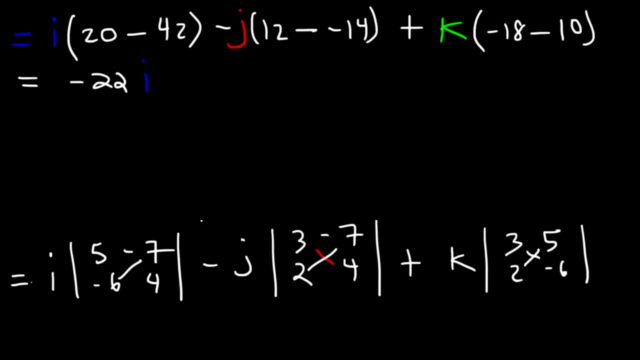 That's 26. And we have a minus in front. So it's going to be negative 26j. 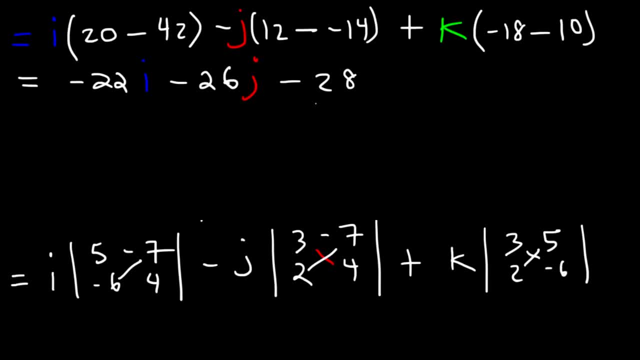 And negative 18 minus 10 is negative 28. So it's negative 28k. 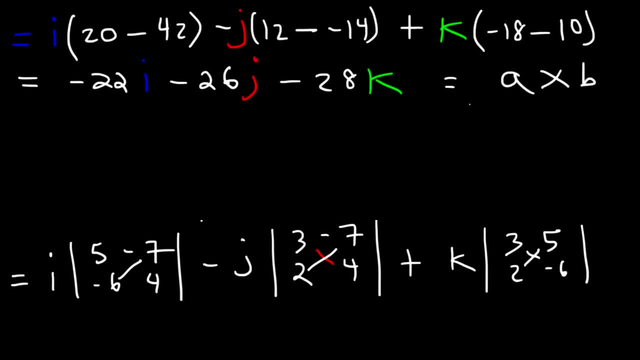 So this is the value of the cross product of a and b. So let's say that c is the cross product of a and b. That means vector c. We can use a little arrow if we want to. 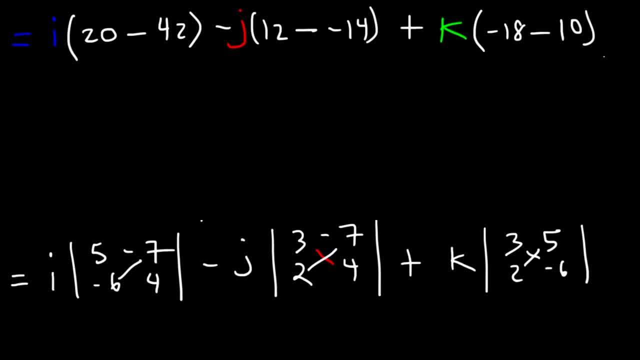 2 times 5 is 10.. So it's minus 10.. Now 20 minus 42.. That's negative 22.. So it's negative 22i And 12 minus negative 14 is like 12 plus 14.. 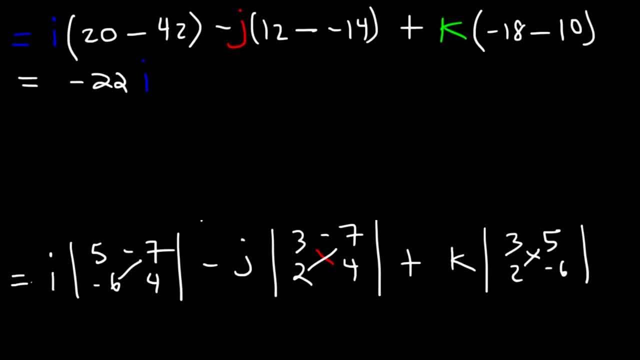 That's 26.. And we have a minus in front, So it's going to be negative 26j And negative 18 minus 10 is negative 28.. So it's negative 28k. So this is the value of the cross product of a and b. 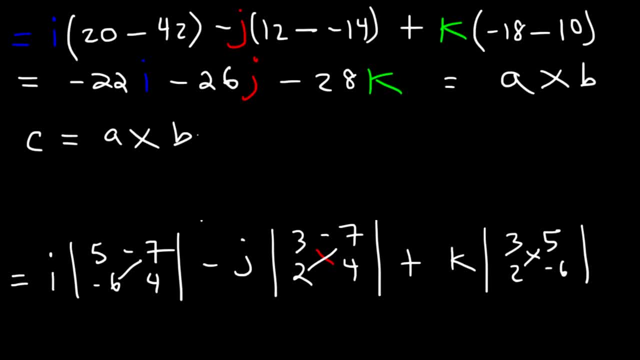 So let's say that c is the cross product of a and b. That means vector c- We can use a little arrow if we want to- Is negative 22i minus 26j minus 28k. So how do we know if we have the right answer or not? 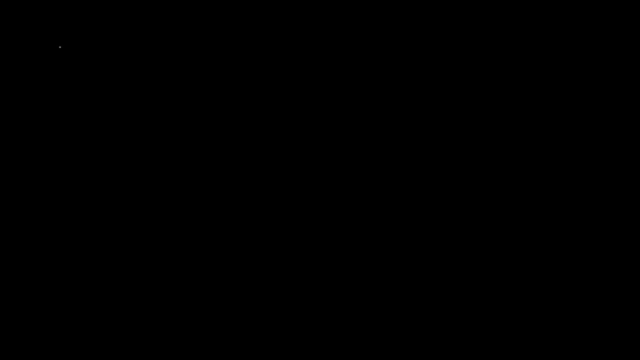 How can we check Now? you need to know that when you have two vectors, let's say vector a and vector b, If you take the cross product of those two vectors, you're going to get another vector, Vector c, that's perpendicular to a and b. 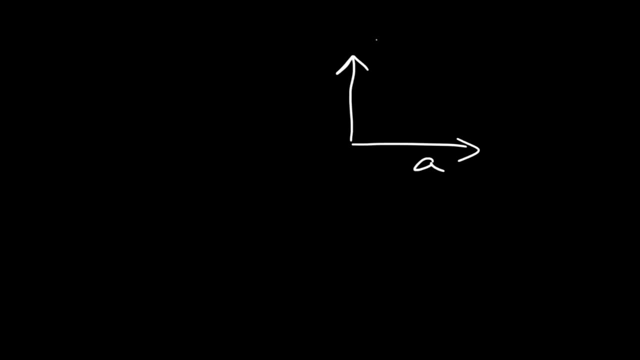 So let's say: if a is perpendicular to b, Let's just draw it. So let's say there's a 90 degree angle, C is going to be perpendicular to both b and vector a. So if a is in the x-axis and let's say b is direct towards the y-axis, c is going to be in the z-axis. 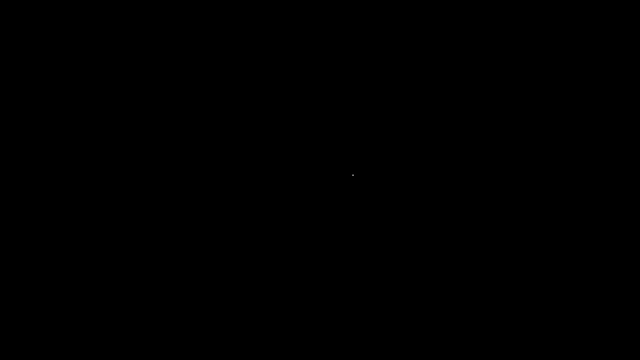 So the new vector, c, is perpendicular to a and b. If you recall, the dot product of two vectors, if they're perpendicular or orthogonal, is equal to 0.. So in this case, since c is the cross product of a and b, 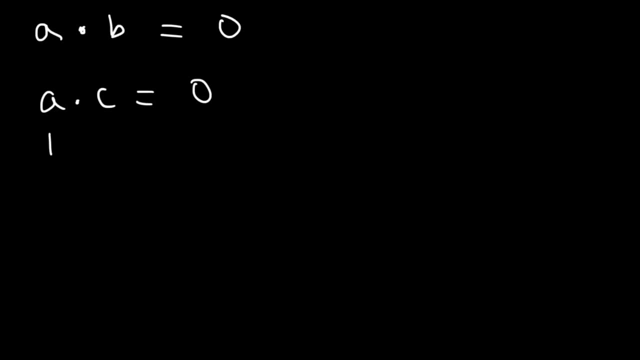 if we take the dot product of a and c, that should be 0.. And the dot product of b and c should be 0. And that's how you can know if you have the right answer or not. So here's the formula. 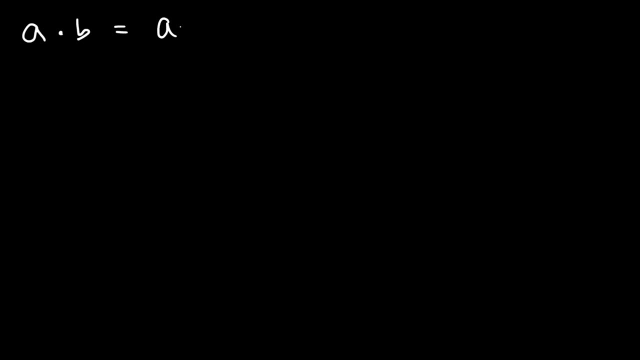 The dot product of a and b is going to be ax times bx Plus ay times by, Plus az times bz. Now we know that vector a is 3i plus 5j minus 7k, So ax is 3, ay is 5, az is negative 7.. 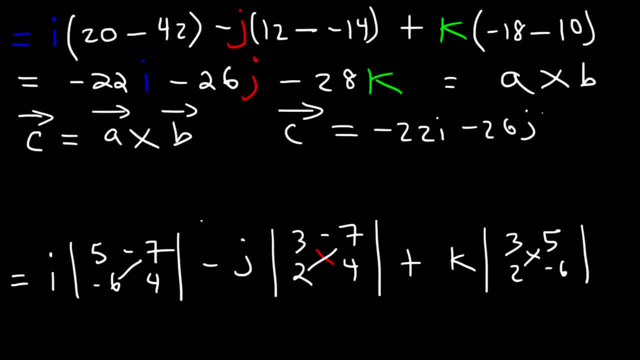 Is negative 22i minus 26j minus 28k. 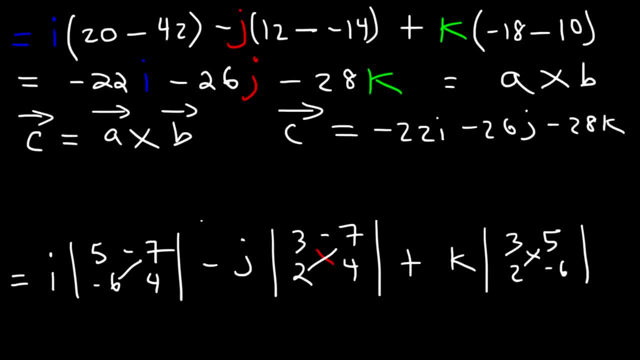 So how do we know if we have the right answer or not? How can we check? 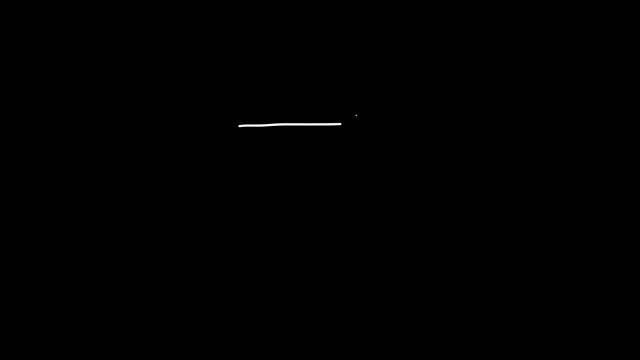 Now, you need to know that when you have two vectors, let's say vector a and vector b, if you take the cross product of those two vectors, you're going to get another vector, vector c that's perpendicular to a and b. So let's say if a is perpendicular to b. Let's just draw it. So let's say there's a 90 degree angle. 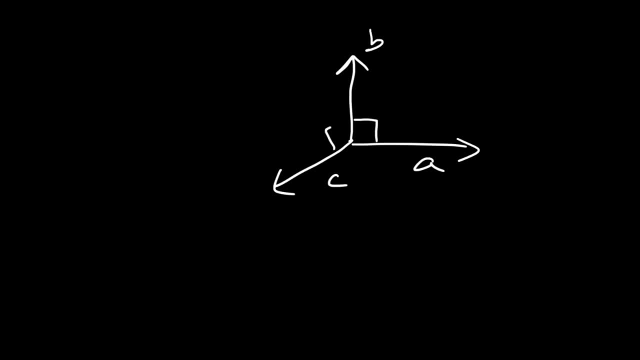 c is going to be perpendicular to both b and vector a. So if a is in the x-axis, and let's say b is direct towards the y-axis, c is going to be in the z-axis. 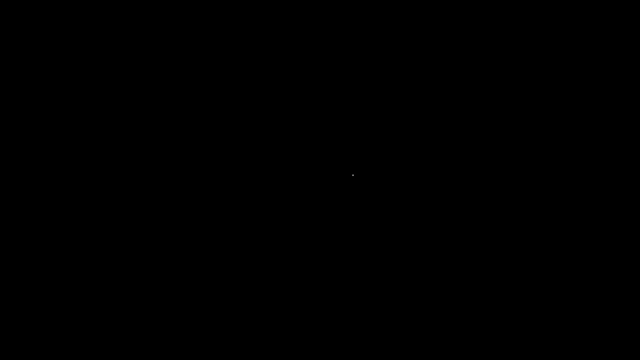 So the new vector c is perpendicular to a and b. If you recall, the dot product of two vectors, if they're perpendicular or orthogonal, is equal to 0. 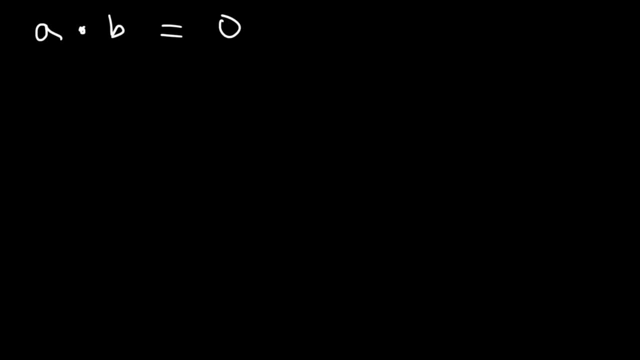 So in this case, since c is the cross product of a and b, if we take the dot product of a and c, that should be 0. And the dot product of b and c should be 0. And that's how you can know if you have the right answer or not. 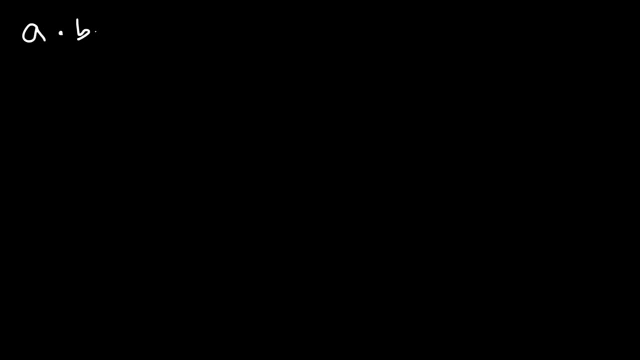 So here's the formula. The dot product of a and b is going to be ax times bx. Plus ay times by. Plus az times bz. 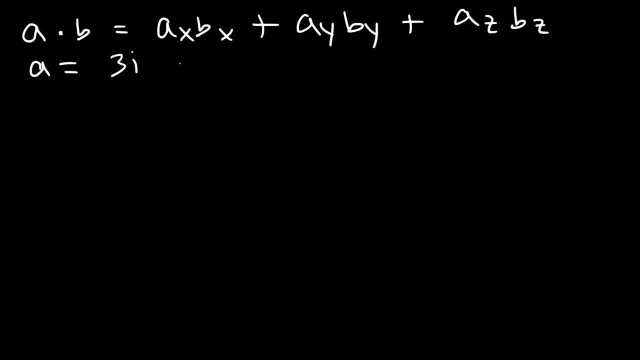 Now we know that vector a is 3i plus 5j minus 7k. So ax is 3, ay is 5, az is negative 7. Vector c, we got it to be negative 22i minus 26j minus 28k. So to find the dot product of a and c, it's going to be ax, cx, plus ay, cy, plus az, cz. So that's 3 times negative 22, plus 5 times negative 26, plus negative 7 times negative 28. 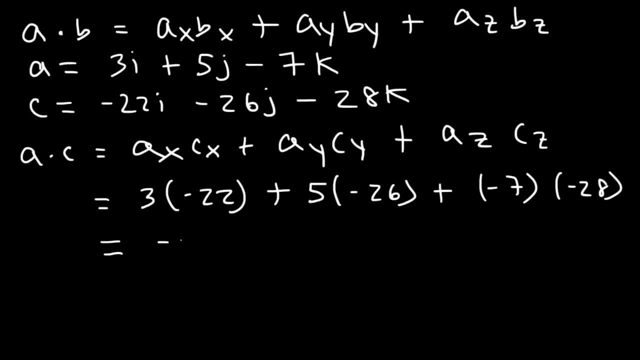 3 times negative 22 is negative 66. 5 times negative 26, that's negative 130. And negative 7 times negative 28, that's positive 196. 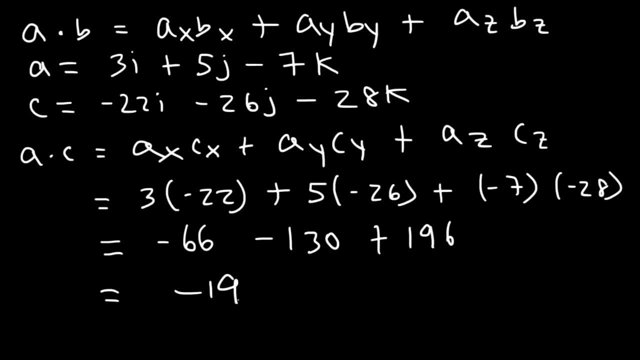 Negative 66 minus 130 is negative 196. So as you can see, this adds up to 0. 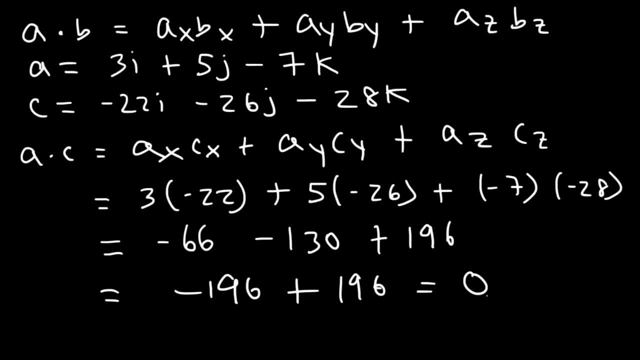 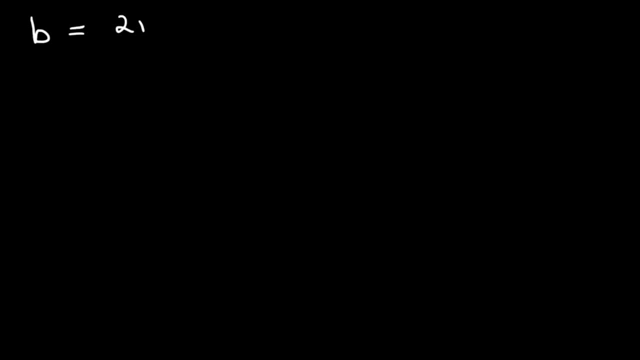 Now let's make sure that the dot product of b and c also is equal to 0. So let's make sure that the dot product of a and c is also equal to 0. So let's make sure that the dot product of b and c is also equal to 0. Vector b is 2i minus 6j plus 4k. 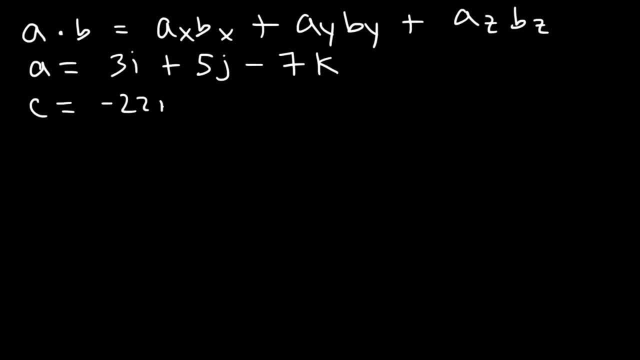 Vector c, we got it to be negative 22i minus 26j minus 28k. So to find the dot product of a and c, it's going to be ax, cx plus ay, cy plus az cz. 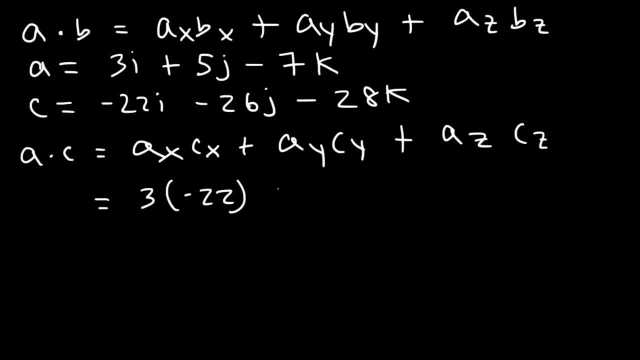 So that's 3 times negative 22, plus 5 times negative 26,, plus negative 7 times negative 28.. 3 times negative 22 is negative 66.. 5 times negative 26,, that's negative 130.. 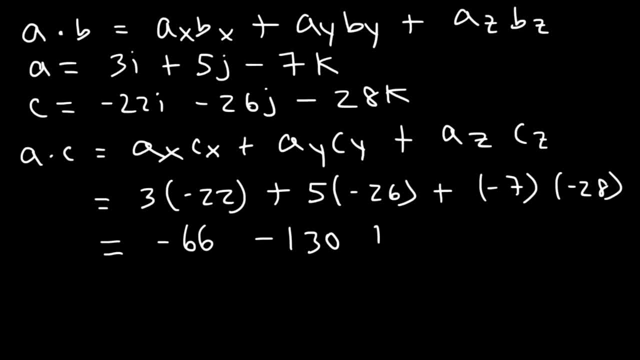 And negative 7 times negative 28,. that's positive 196.. Negative 66 minus 130 is negative 196.. So, as you can see, this adds up to 0.. Now let's make sure that the dot product of b and c also is equal to 0.. 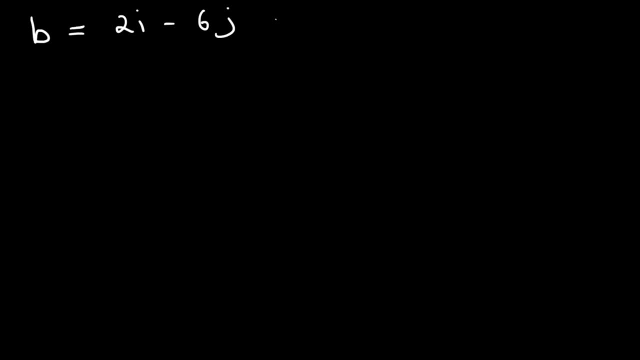 Vector b is 2i minus 6j plus 4k And vector c- we know it's a negative- 22i minus 26j minus 28k. So let's find the dot product of b and c. So it's going to be bx times cx plus by times cy. 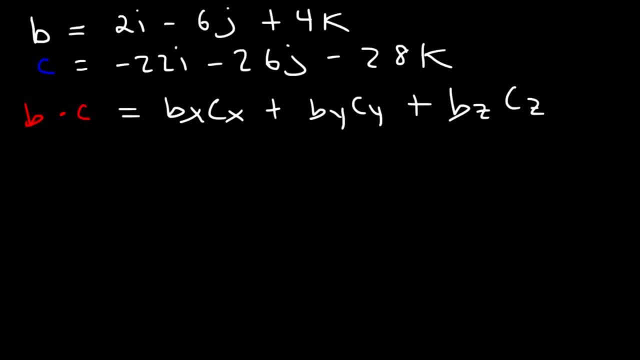 So bx is 2, cx is negative 22. By that's negative 6. Cy is negative 26.. Bz is 4. Cz is negative 28. So 2 times negative 22,. that's negative 44.. 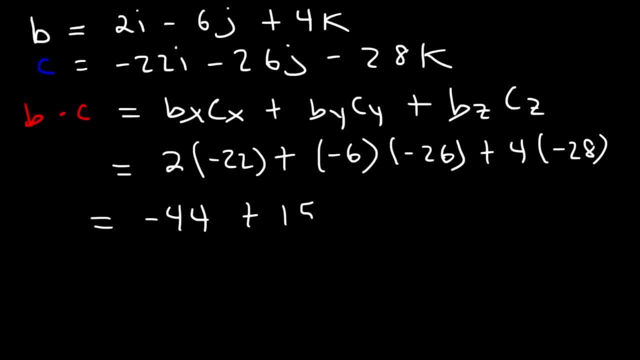 And negative 6 times negative 26,. that's positive 156.. 4 times negative: 28.. That's negative 112.. Negative 44 plus 156 is positive 112.. So, as you can see, this is 0.. So that's how you can tell if you have the right answer. 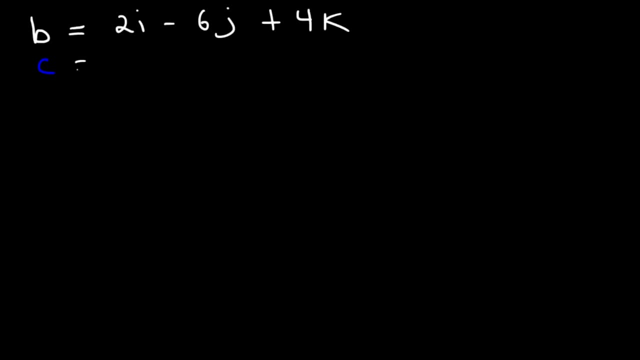 And vector c, we know it's negative 22i minus 26j minus 28k. So let's find the dot product of b and c. So it's going to be bx times cx plus by times cy. So bx is 2, cx is negative 22. By, that's negative 6. Cy is negative 26. Bz is 4. Cz is negative 28. So 2 times negative 22, that's negative 44. 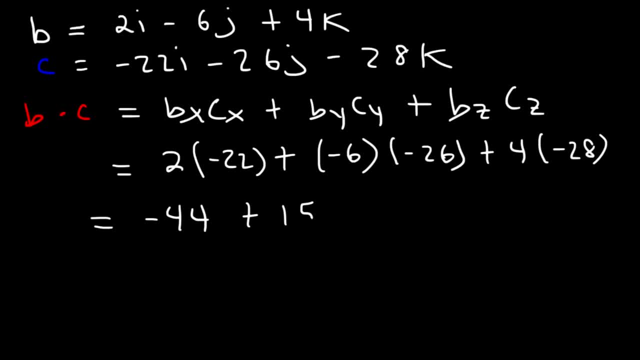 And negative 6 times negative 26, that's positive 156. 4 times negative 28. That's negative 112. 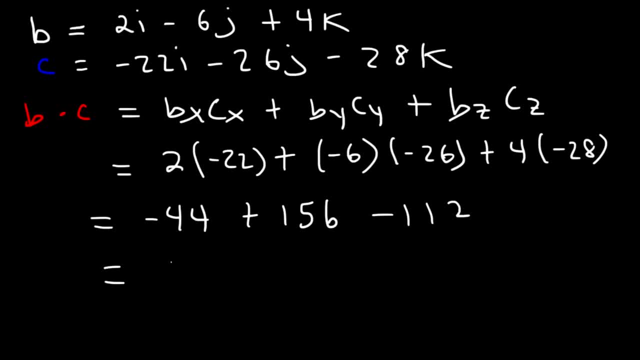 Negative 44 plus 156 is positive 112. So as you can see, this is 0. 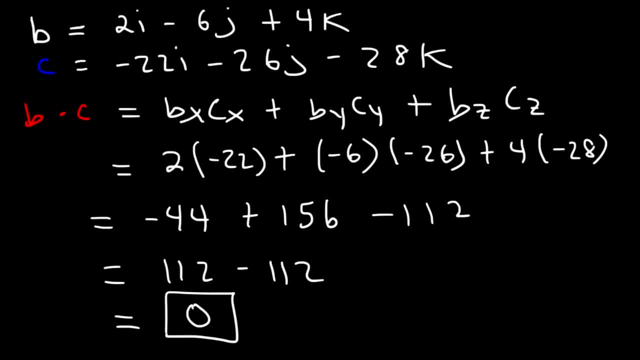 The answer that you get if you find the dot product, let's say with vector c and vector a or vector b, both should equal 0. Because the new vector is orthogonal or perpendicular 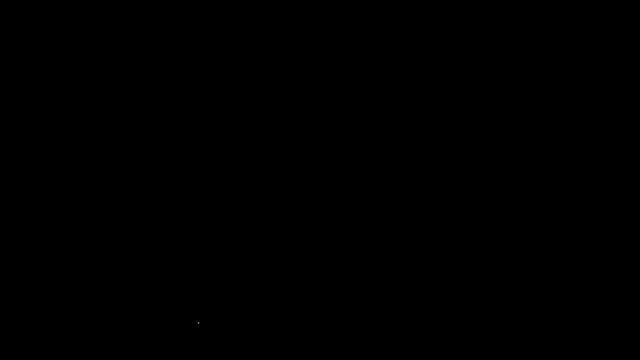 to the two vectors that created it. Now let's work on another example. So let's say if vector A has the components 5, negative 4, and 3, and vector B is negative 7 to negative 8. Find a cross product of vectors A and B, and let's call that answer vector C, which we know is perpendicular to both A and B. So if you see it in this form, just keep in mind A is the same as 5i minus 4j plus 3k, and B is basically negative 7i plus 2j minus 8k. So the work is going to be the same. Let's write this in a 3x3 matrix. So let's start with a 3x3 matrix. 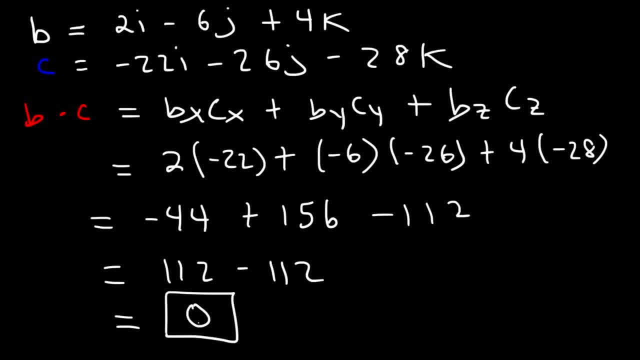 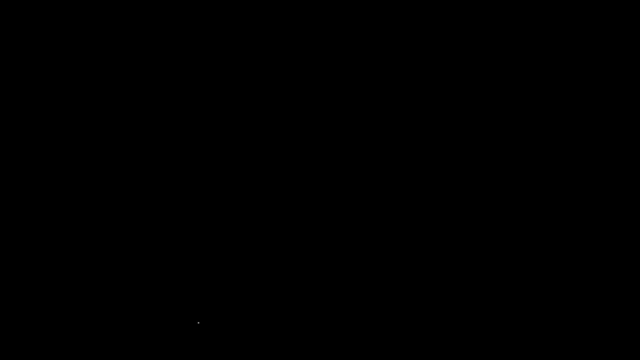 The answer that you get if you find the dot product, let's say with vector c and vector a or vector b, both should equal 0. Because the new vector is orthogonal or perpendicular To the two vectors that created it. Now let's work on another example. 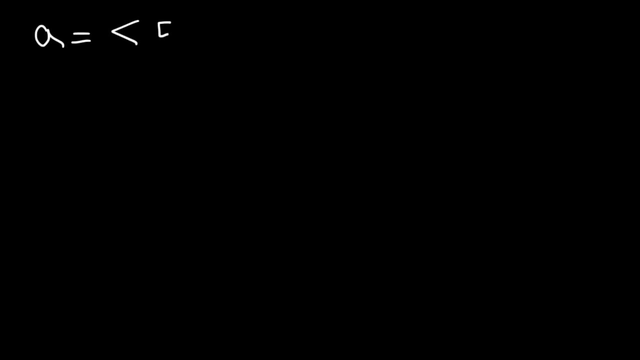 So let's say if vector a has the components 5,, negative 4, and 3. And vector b is negative, 7 to negative 8. Find the cross product of vectors a and b And let's call that answer vector c. 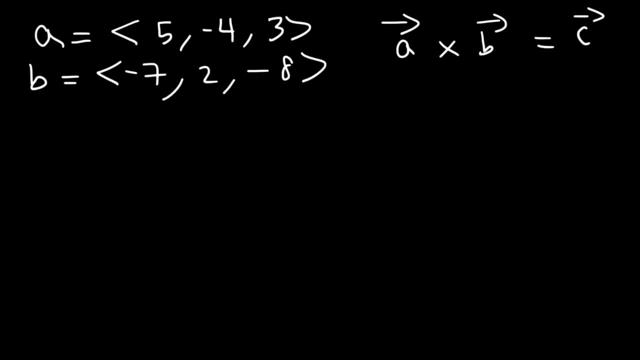 Okay, Which we know is perpendicular to both a and b. So if you see it in this form, just keep in mind a is the same as 5i minus 4j plus 3k And b is basically negative: 7i plus 2j minus 8k. 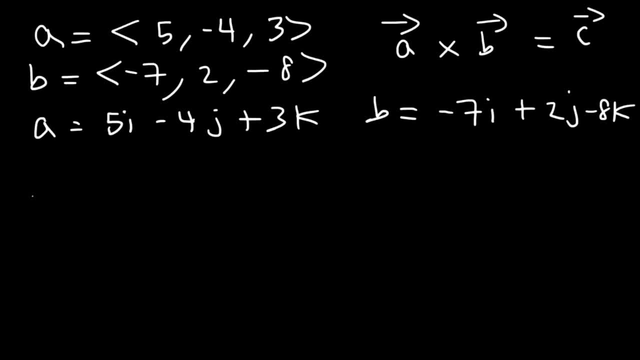 So the work is going to be the same. Let's write this in a 3 by 3 matrix. So let's start with i, j, And then the first vector is a. That's going to be in the second row. So that's 5, negative, 4, 3.. 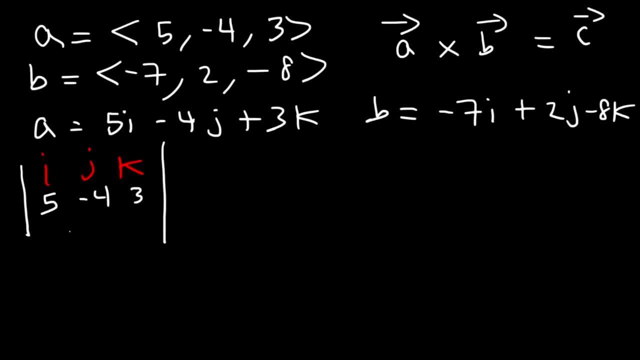 And the second vector is going to be in the third row And that's negative 7, 2, negative 8.. So go ahead and calculate the cross product. So first let's start with i, which is in the first row, first column. 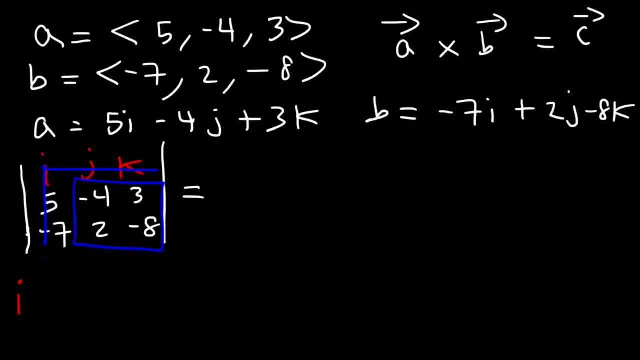 And that's going to produce the 2k: 2 by 2 matrix negative 4, 3, 2, negative 8. And then it's going to be minus vector j, Or not vector j, but like component j. 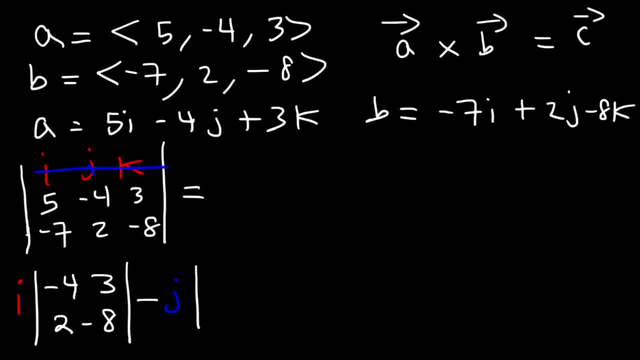 And that is in the first row, second column. So that's going to leave behind 5, negative 7, and 3, negative 8.. And then plus k. k is in the first row, third column. So it's going to leave behind 5, negative 7, negative 4, and 2.. 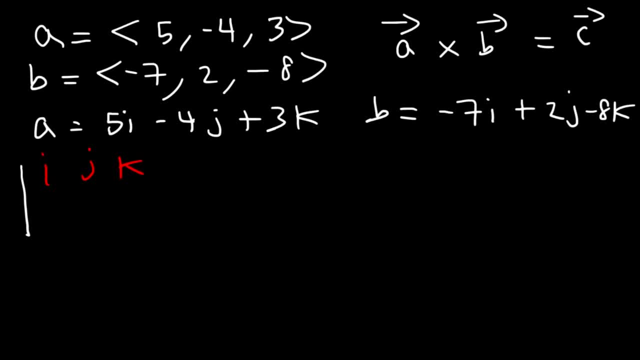 Let's start with i, j, k, and then the first vector is A. That's going to be in the second row. So that's 5, negative 4, 3, and the second vector is going to be in the third row, and that's negative 7, 2, negative 8. So go ahead and calculate the cross product. So first let's start with i, which is in the first row, first column, and that's going to produce the 2x2 matrix, negative 4, 3, 2, negative 8. And then it's going to be minus vector j, or not vector j, but like component j, and that is in the first row, second column. So that's going to leave behind 5, negative 7, and 3, negative 8. And then plus k. k is in the first row, third column. So it's going to leave behind 5, negative 7, negative 4, and 2. 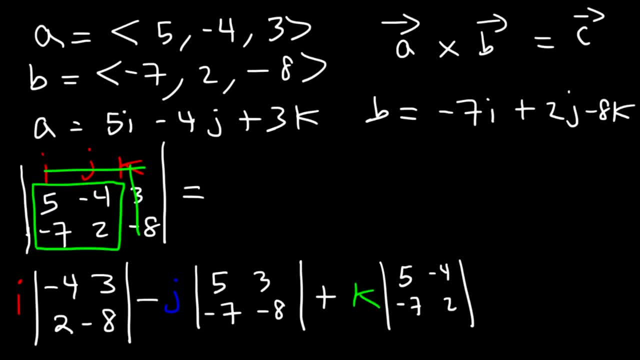 So that's going to leave behind 5, negative 7, negative 4, and 2. So now let's go ahead and evaluate the 2x2 determinants. 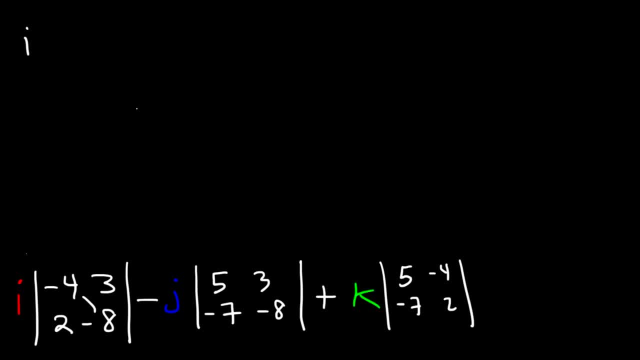 So it's i, and then it's negative 4 times negative 8, that's 32, minus 2 times 3, which is 6. And then minus j, 5 times negative 8, that's negative 40, minus negative 7 times 3, which is negative 21. Plus k, and then 5 times 2 is 10, minus negative 7 times negative 4 is positive 28. So 32 minus 6 is 26. Here we have negative 40 plus 20, because we have two negative signs, I mean plus 21. Negative 40 plus 21, that's negative 19. And 10 minus 28 is negative 18. So that's negative 19. 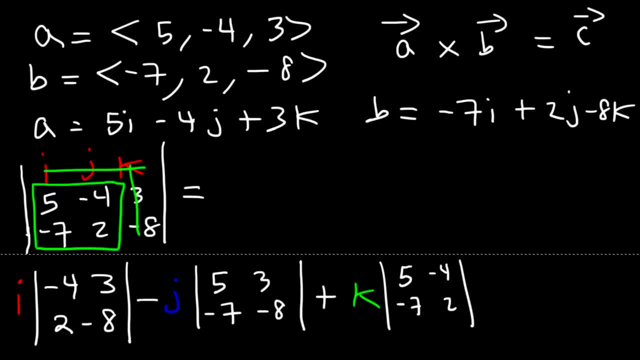 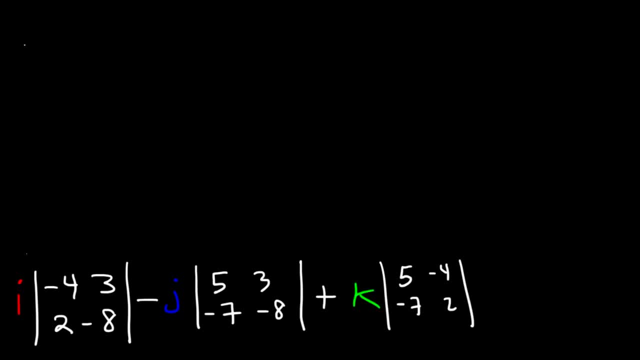 So now let's go ahead And evaluate the 2 by 2 determinants. So it's i, And then it's negative 4 times negative 8. That's 32.. Minus 2 times 3,, which is 6.. 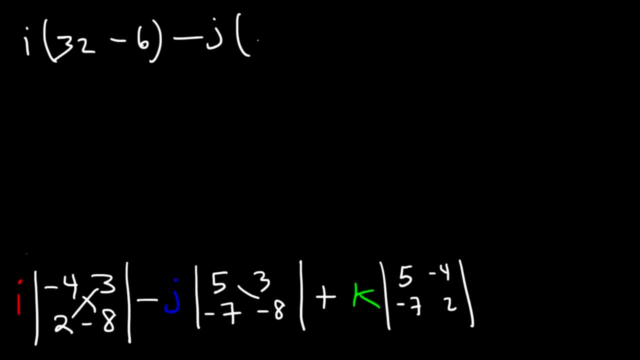 And then minus j, 5 times negative 8,, that's negative 40. Minus negative 7 times 3,, which is negative 21.. Plus k And then 5 times 2 is 10.. Minus negative 7 times negative, 4 is positive 28.. 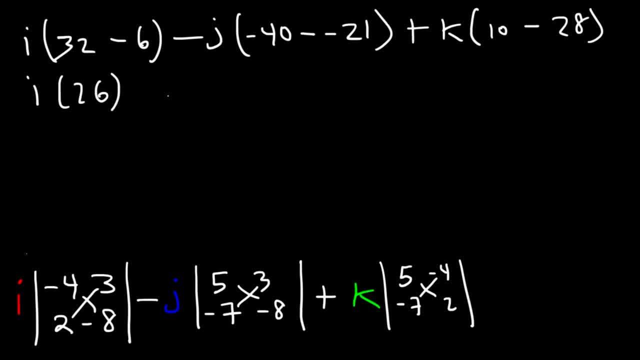 So 32 minus 6 is 26.. Here we have negative 40 plus 20, because we have two negative signs. I mean plus 21.. Negative 40 plus 21,. that's negative 19.. And 10 minus 28 is negative 18.. 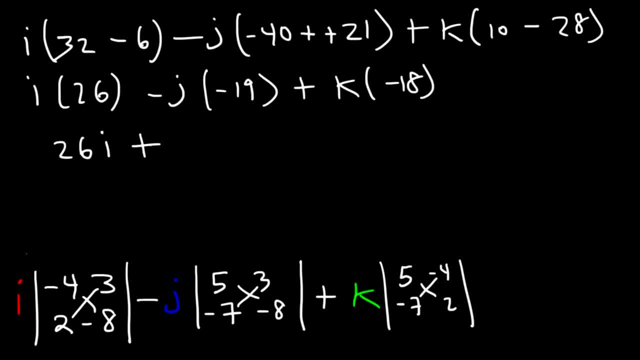 So this is going to be 27.. So this is going to be 26i plus 19j minus 18k. So that's the new vector. That's how you can find it. Now, just to make sure that we have the right value. 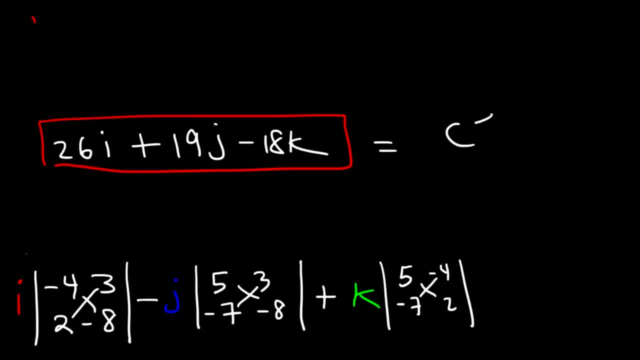 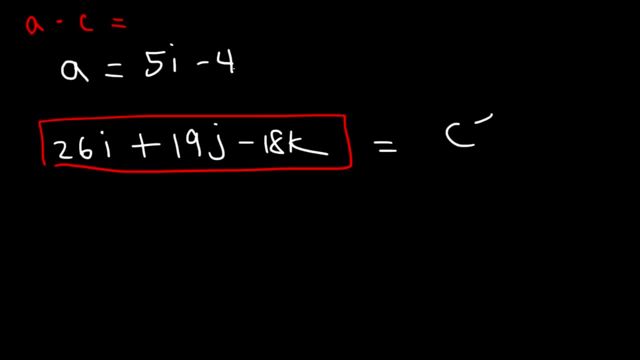 Now, if you recall, vector A is 5i minus 4j plus 3k, So the dot product of A and C is going to be Ax, Cx plus Ay, Cy and then Az times Cz. So Ax is 5,, Cx is 26,, Ay is negative 4,, Cy is 19, and Az is 3, Cz is negative 18.. 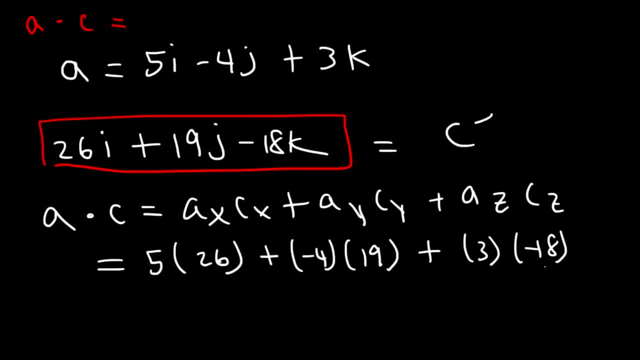 5 times 26,, that's 130.. And then we have negative 4 times 19,, which is negative 76, and 3 times negative 18,, that's negative 54.. 130 minus 76 is 54.. 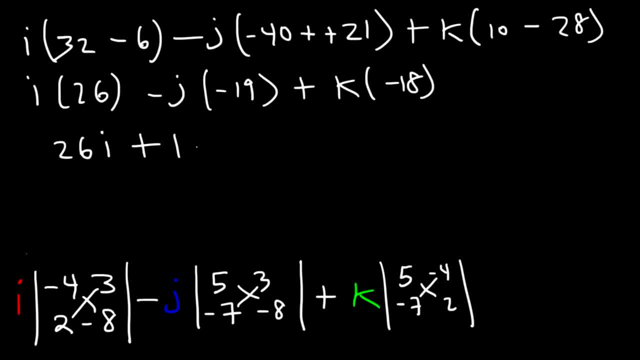 So this is going to be 26i plus 19j minus 18k. So that's the new vector. That's how you can find it. 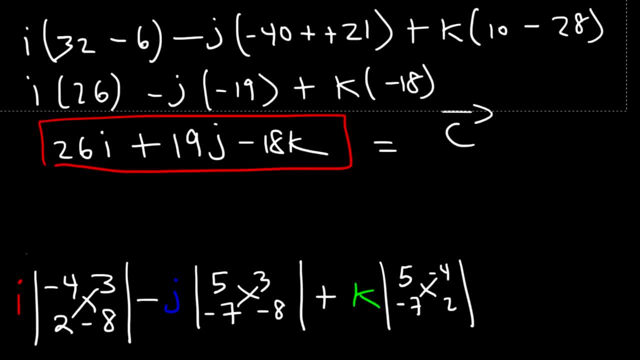 Now, just to make sure that we have the right value, let's test the dot product of a and c. Let's make sure it's equal to 0. 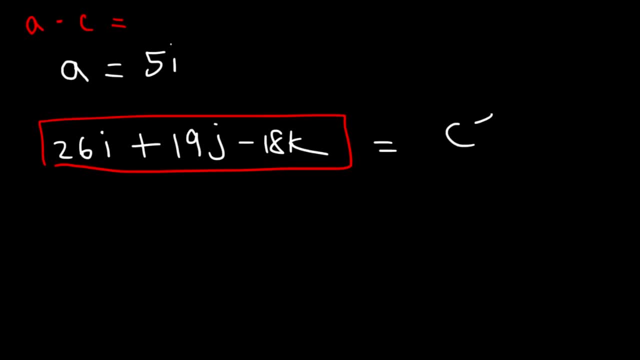 Now, if you recall, vector a is 5i minus 4j plus 3k. So the dot product of a and c is going to be ax, cx, plus ay, cy, and then az times cz. 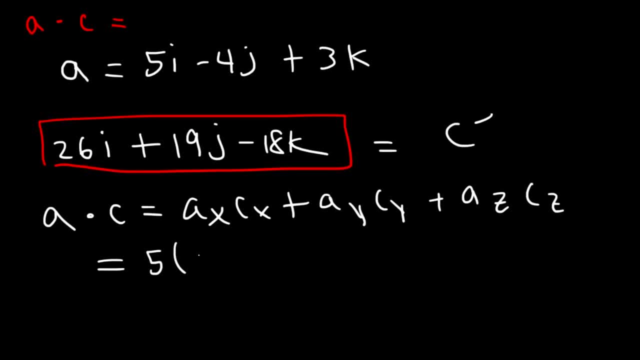 So ax is 5, cx is 26. 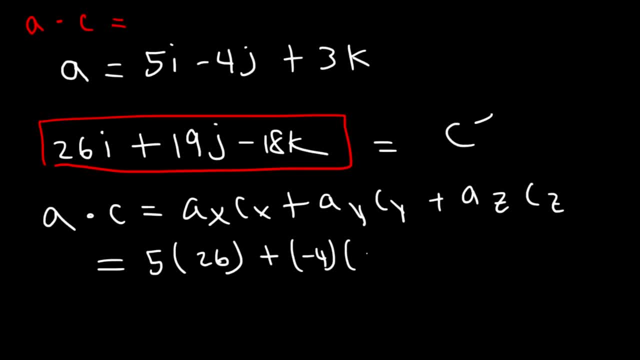 Ay is negative 4, cy is 19. And az is 3, cz is negative 18. 5 times 26, that's 130. 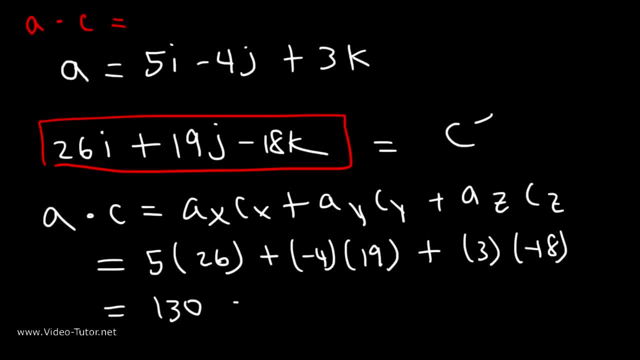 And then we have negative 4 times 19, which is negative 76. And 3 times negative 18, that's negative 54. 130 minus 76 is 54. So it's 54 minus 54, which is 0. 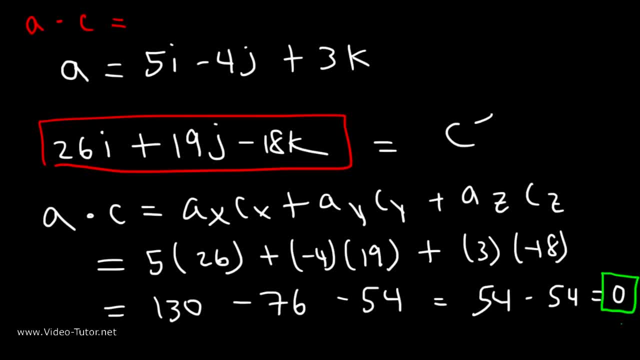 So the fact that a and c are orthogonal means that this is the right answer. And then just to confirm, just to double check, you can make sure that the dot product of vector b and c, if that's equal to 0, then you know that you have the right answer. This is the cross product of a and b. 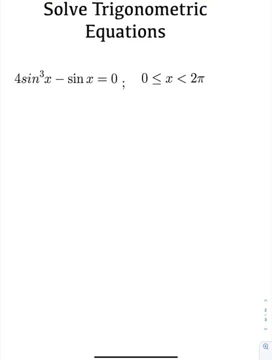 All right, we're going to be doing a quick example of solving trig equations. So when you're going to solve trig equations, the first thing you want to be able to do is try to factor this in any way you can. You can see, with this equation here we can factor the sine of x. So I'm going to go ahead and 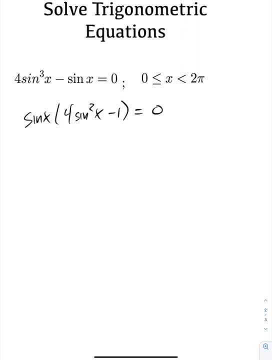 do that, We now have the product of two expressions equals zero. So the only way that this can be zero here either the sine of x is going to have to be zero, or with a four sine squared x minus one must be equal to zero. So we end up generating here three equations: either the sine of x is zero.